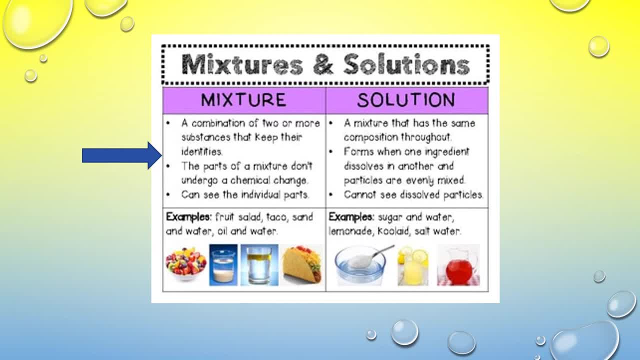 don't undergo a chemical change and you can see the individual parts. Examples are things like fruit salad, tacos, sand and water. oil and water. A solution is a mixture that has the same composition throughout and it forms when one ingredient dissolves in another and particles. 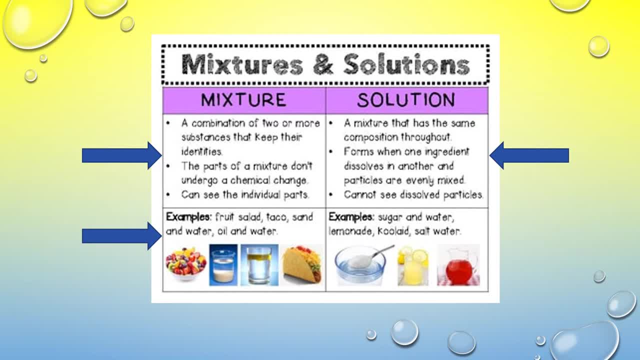 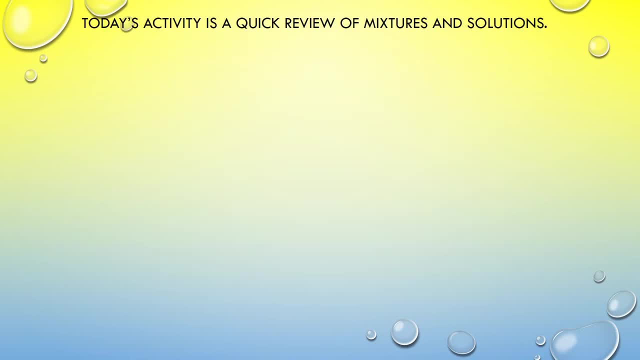 are evenly mixed, You cannot see the dissolved particles. Examples are things like sugar and water, lemonade, Kool-Aid and salt water. Today's activity is a quick review of mixtures and solutions. The exercises for this lesson are cross crawls, which are going to be mixtures. 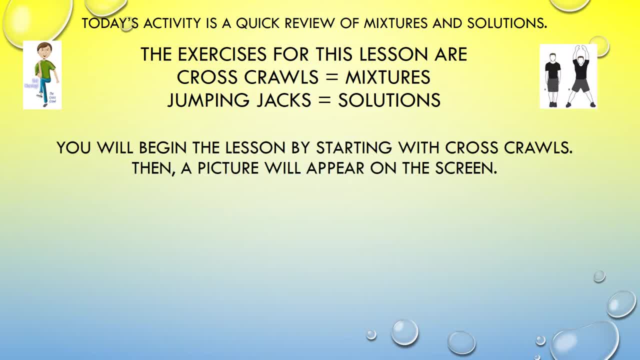 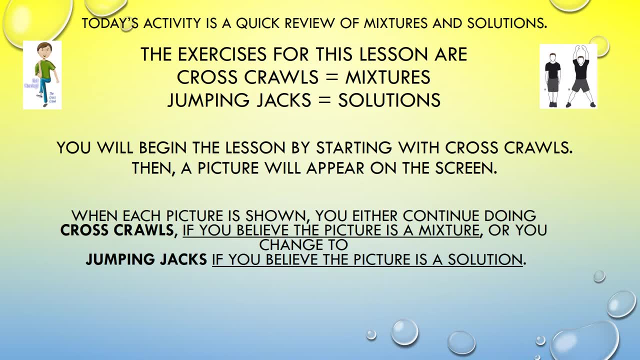 and jumping jacks, which will be solutions. You will begin the lesson by starting with cross crawls, then a picture will appear on the screen. When each picture is shown, you either continue doing cross crawls if you believe the picture is a mixture, or you change to jumping jacks if you 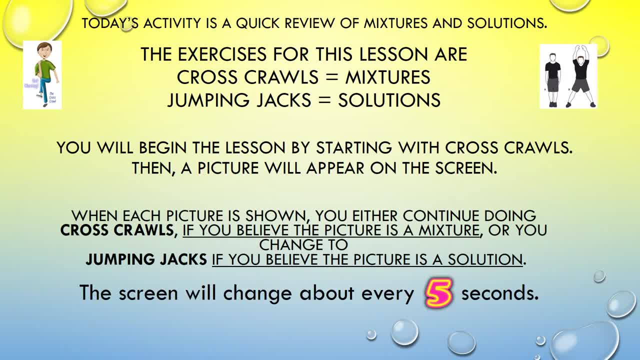 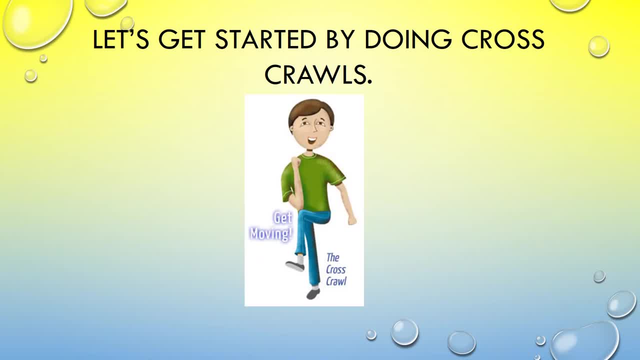 believe the picture is a solution. The screen will change about every five seconds. Let's get started by doing cross crawls. When the next screen appears, you will continue to do cross crawls if you think it is a mixture, but if it's a solution, you will change to jumping jacks. 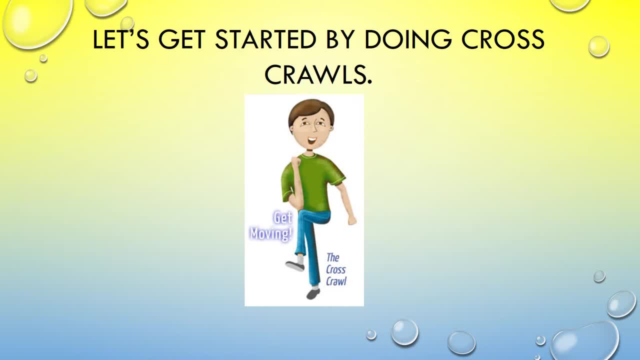 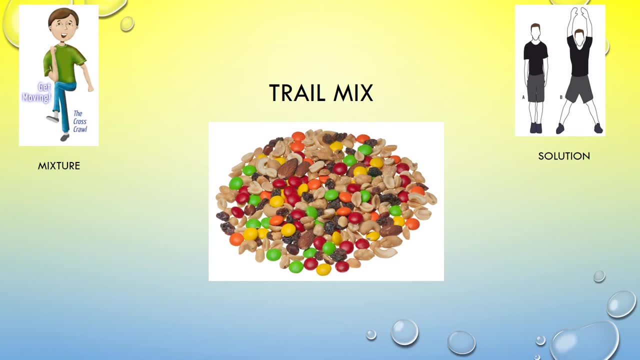 Ready, Let's go. Here's our first one trail mix. You should still be doing either cross crawls or change to jumping jacks. if you think this is a solution, Keep it up. You should be doing cross crawls. Keep going with cross crawls until the next picture appears. This picture is Gatorade. 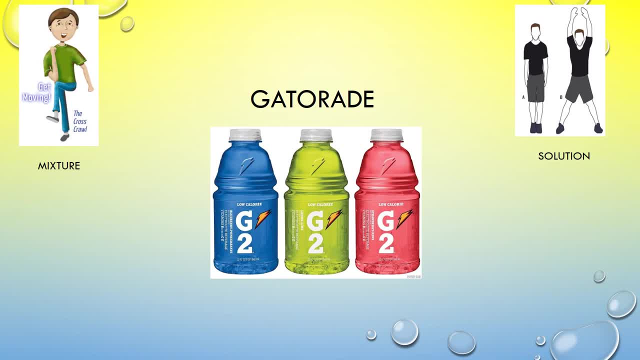 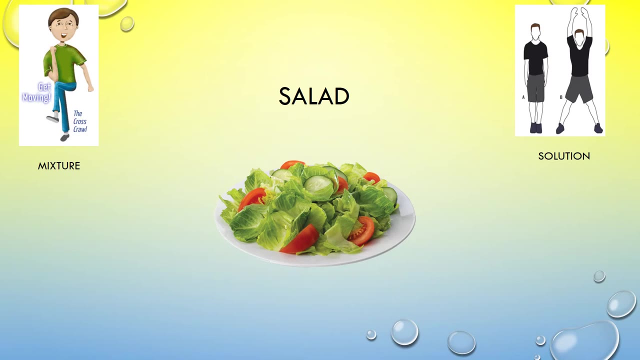 Either you're doing cross crawls or you're doing jumping jacks. Keep on going. All right, If you're doing jumping jacks, you are correct. Keep doing jumping jacks until the next screen appears. Here we have a salad. Will you continue doing jumping jacks or will you switch back to? 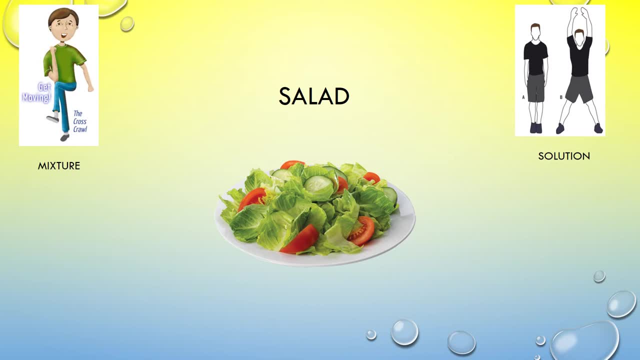 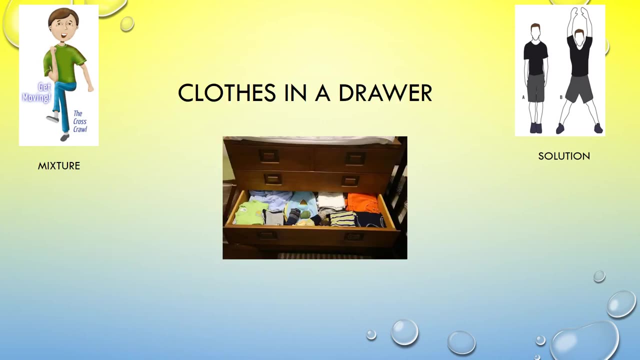 cross crawls. Okay, you should have switched back to cross crawls. Our next one is clothes in a drawer. Will you do cross crawls for mixture or jumping jacks for solution? These are a mixture, so you should have been doing cross crawls. Keep on going until the next. 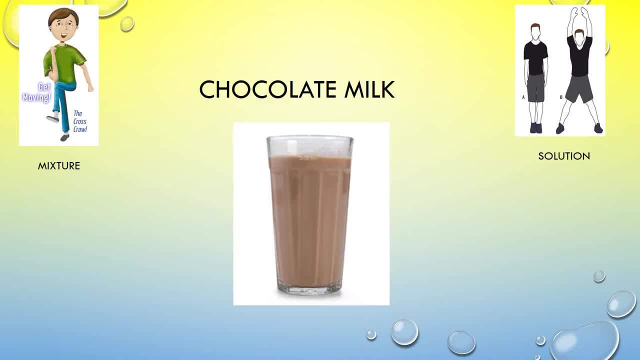 picture appears. Our next item is chocolate milk Cross crawls for mixture. jumping jacks for solution. Okay, it is a solution, so jumping jacks was the answer. Here we have iced tea. Will you continue to do jumping jacks or switch to cross crawls? 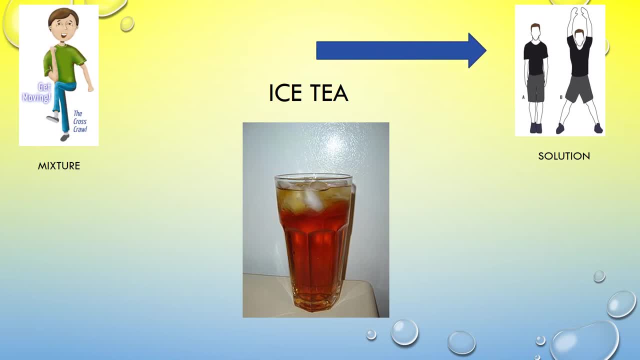 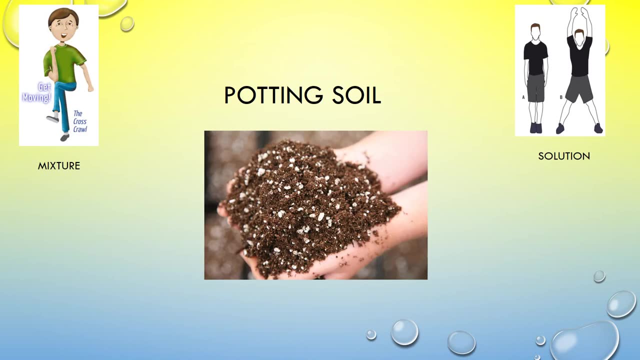 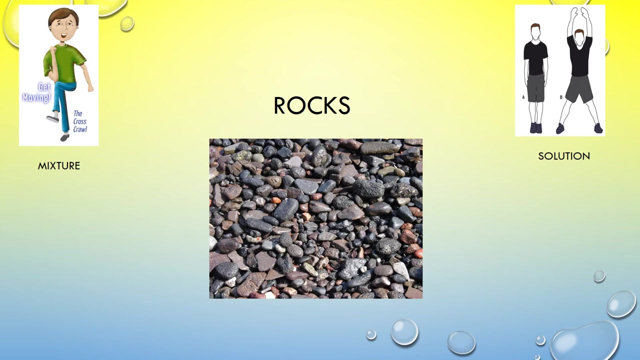 Ice tea is a solution. Keep on going until the next screen appears. Our next one is potting soil. Will you continue doing jumping jacks or will you change to cross crawls? Potting soil is a mixture, so cross crawls was the correct answer. Here we have a bunch of rocks. Mixture or solution. 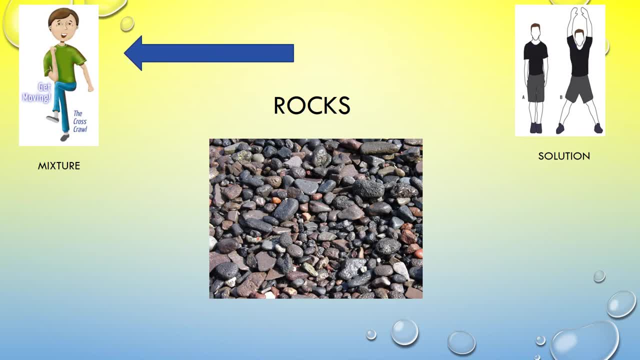 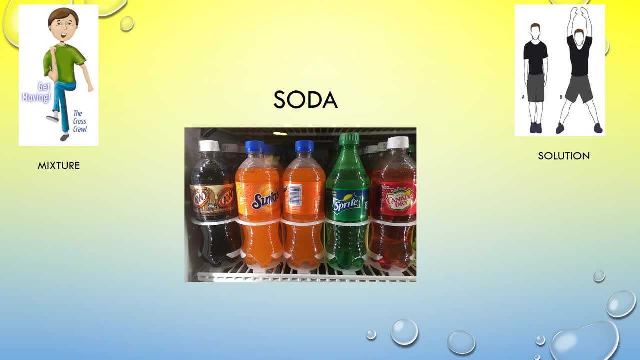 It's a mixture, so cross crawls was the answer. Keep going. We now have soda. Will you change to jumping jacks or continue with cross crawls? Hopefully you change to jumping jacks, since soda is a solution. Hopefully you're still going. Here's our next one: salt water. Will you continue? 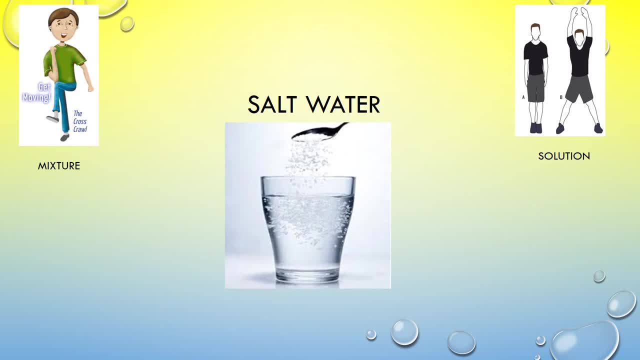 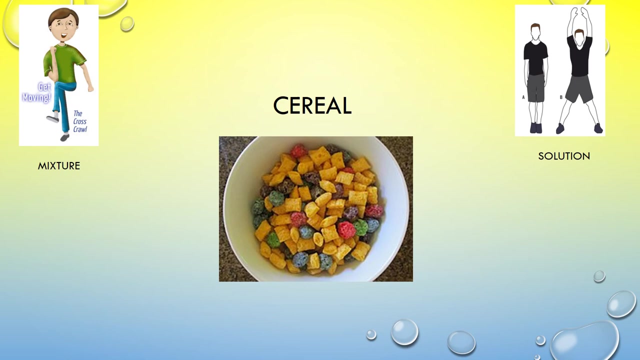 to do jumping jacks or change to cross crawls 水, But We've got a lot of water, so that's a solution. Here we have cereal. Will you continue with jumping jacks? or change to cross crawls? kort, Johnny is dreamer. Still he does water arenas every day. 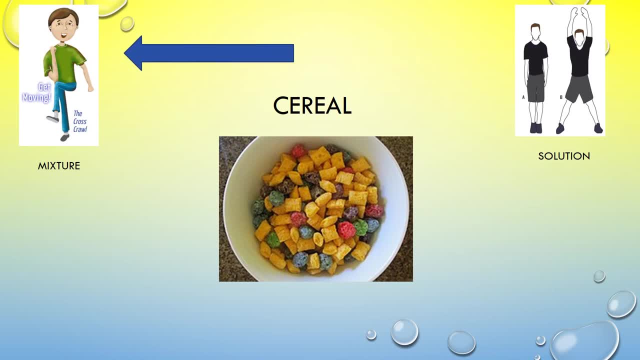 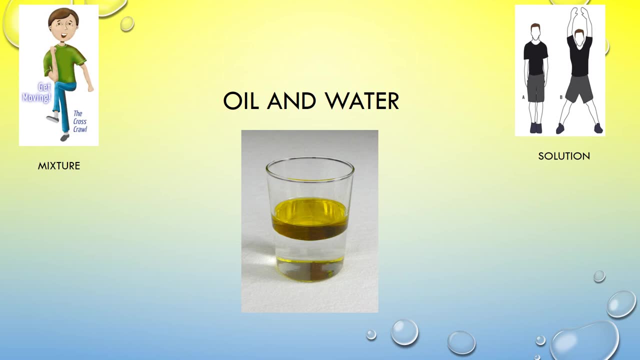 Keep watching for new sales videos before shopping. All right, this is a mixture. Get ready for our last one. keep going. Our last one is oil. waterBabyiley asks: Will it be a mixture, Will it be a solution? מא. 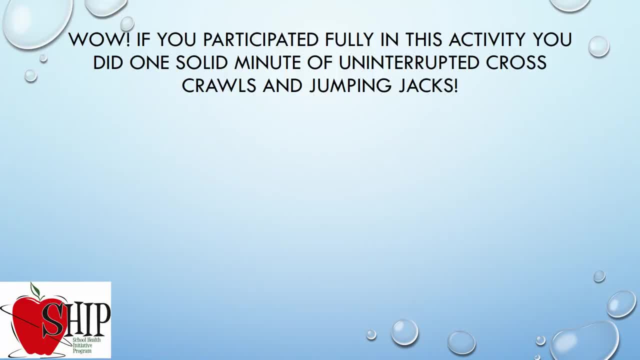 cross-crawls. You can take a break now. Wow, if you participated fully in this activity, you did one solid minute of uninterrupted cross-crawls and jumping jacks. You're probably out of breath. And just remember that there is a property difference between mixtures and solutions. 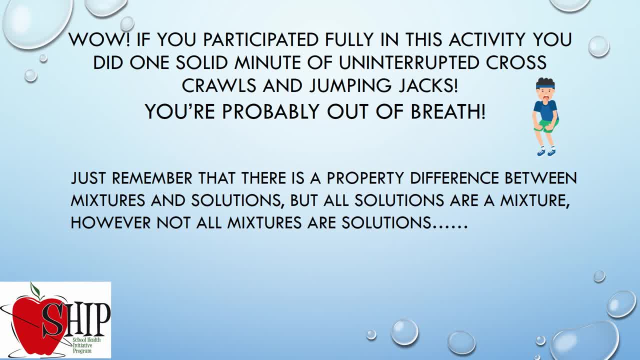 but all solutions are a mixture. However, not all mixtures are solutions. Have a great one.